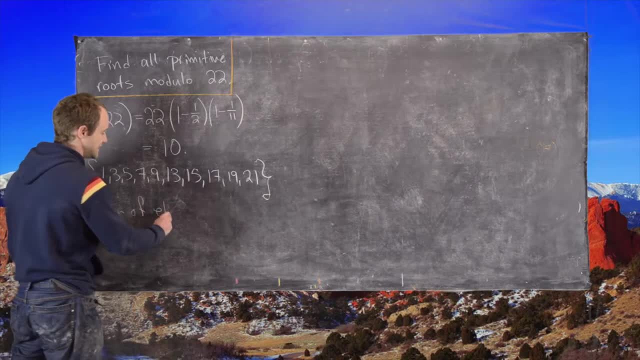 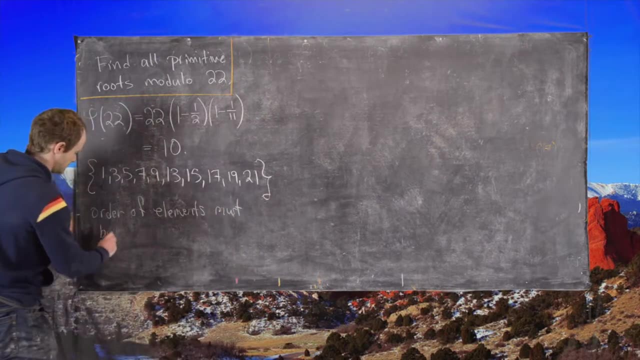 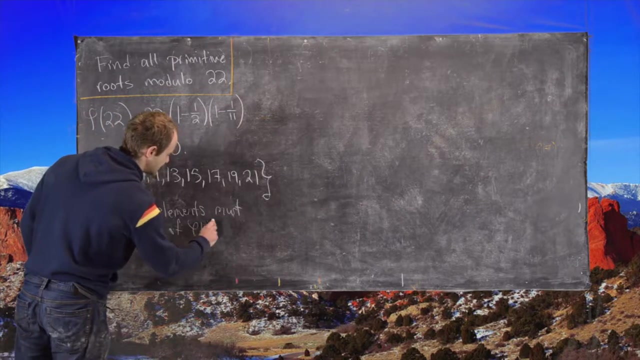 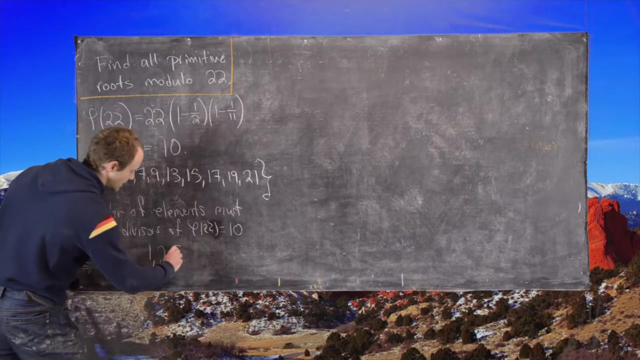 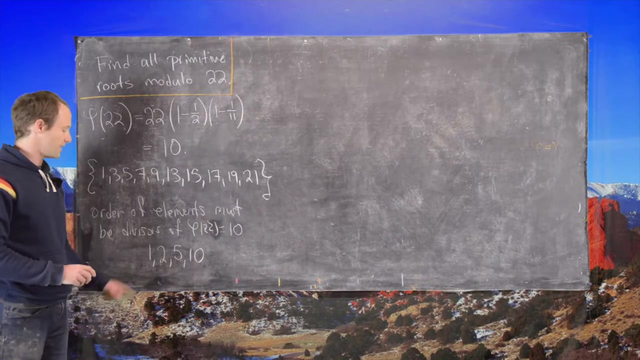 of these elements must be divisors of phi of 22, which equals 10, right? so the possible orders, in other words, are 1,, 2,, 5, and 10. so those are the only exponents that we really need to check. we don't have to check anything other than something to the first power. 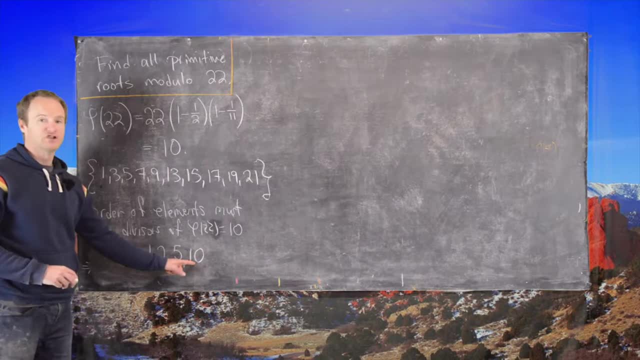 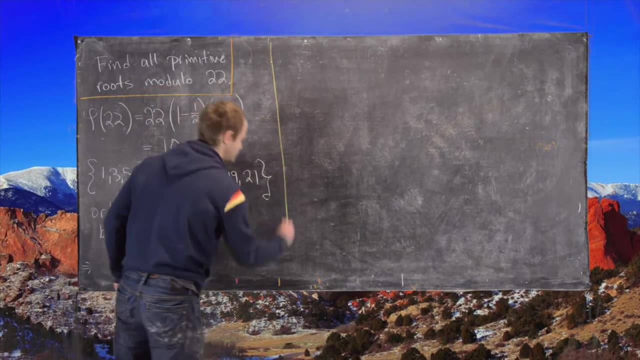 squared to the fifth power, and then we won't have to check to the tenth power because we will have already checked everything before. okay, so let's get going. so let's start with 3, because obviously 1 to the first is 1, so the order of 1 is 1. 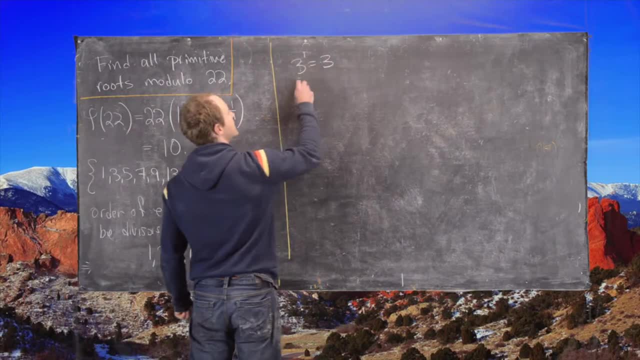 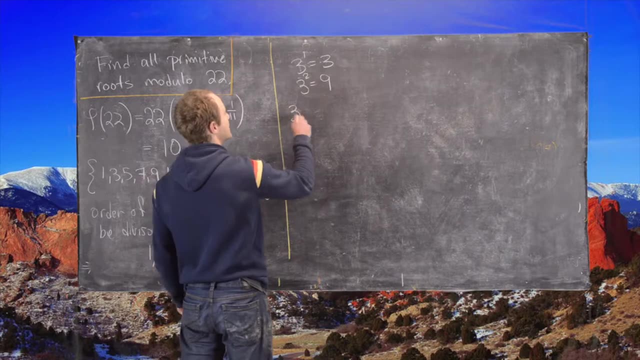 so now we have: 3 to the first is equal to 3. 3 squared is equal to 9. so 9 is obviously not equal to 1. then 3 to the fifth. so I want to use just everything previous. so I want to use just everything previous. so I want to use just everything previous. 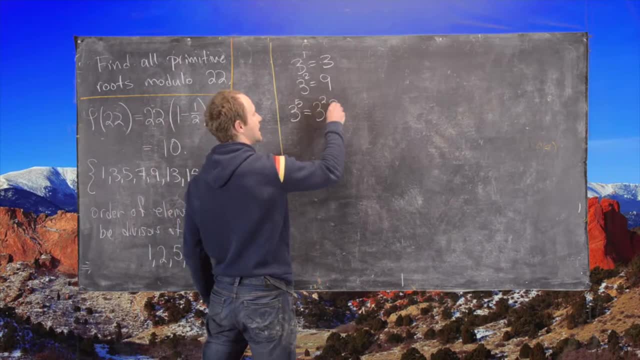 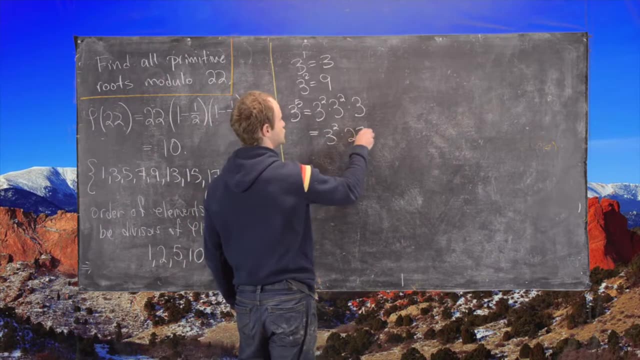 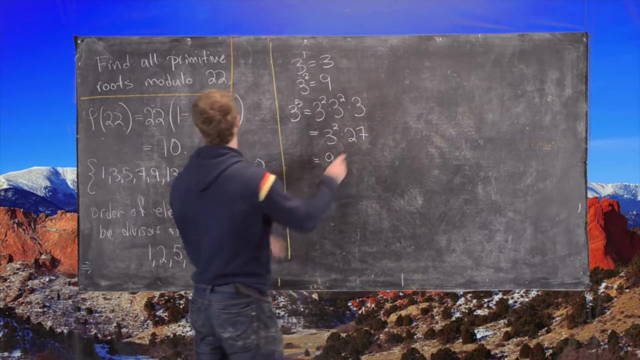 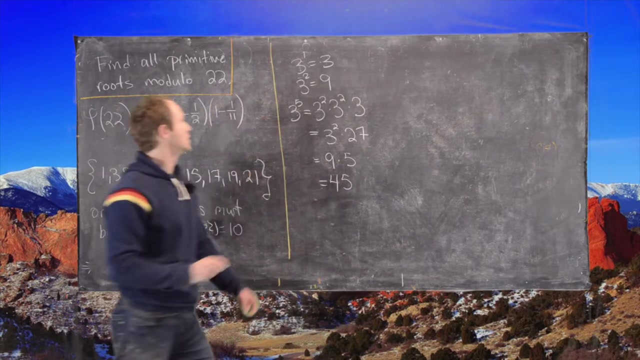 so notice that will be 3 squared times 3 squared times 3. so notice that gives us 3 squared times 27. great, but that gives us 9 times now. 27 modulo 22 is 5, so that gives us 45, which is one more than 44. 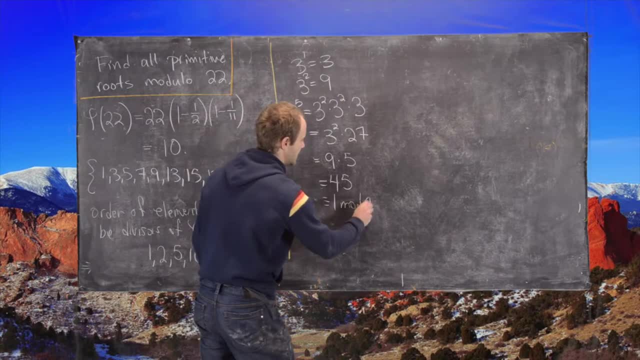 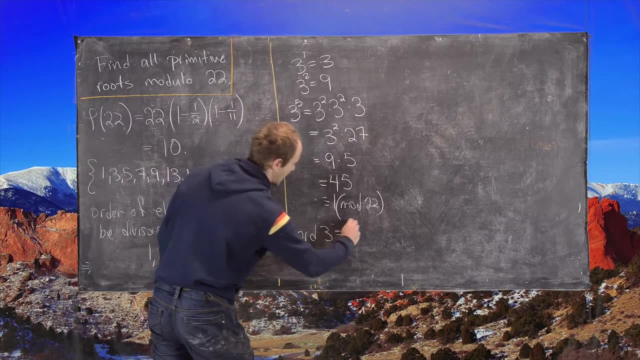 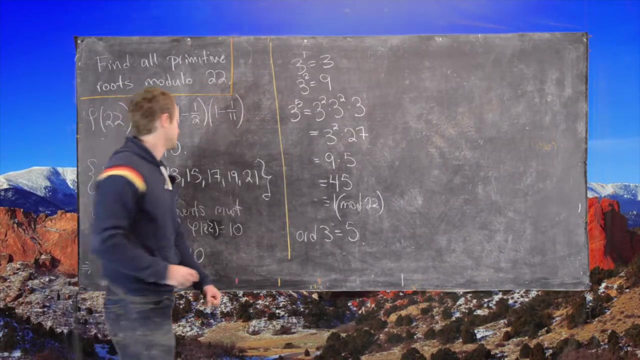 so that means that this is congruent to 1 into mod 22, 2, 9, 3 and so on. we got that the order of 3 is equal to 5. great, so the order of 3 is equal to 5. so it is not a primitive root. 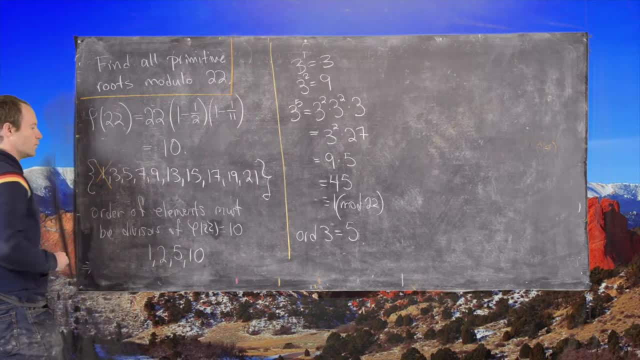 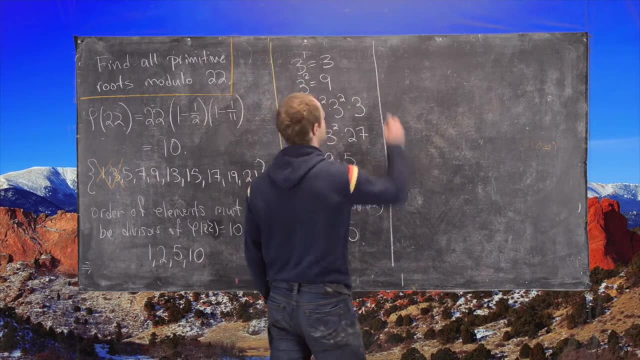 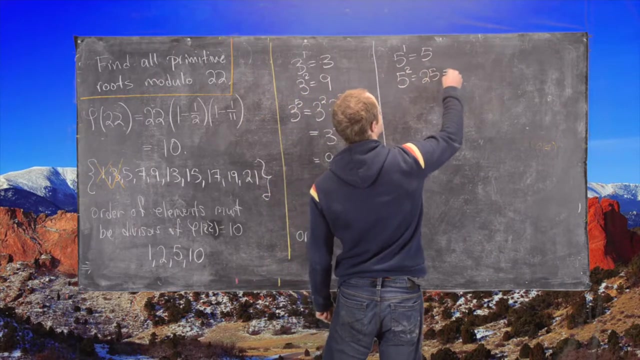 so here we can cross this out as we can also. 1 is not a primitive root. 3 is not a primitive root. let's move on to 5. so we have 5 to the first is equal to 5. 5, 5 squared is equal to 25, which is equal to. 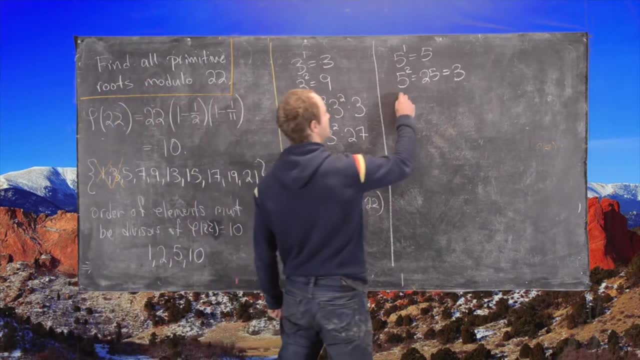 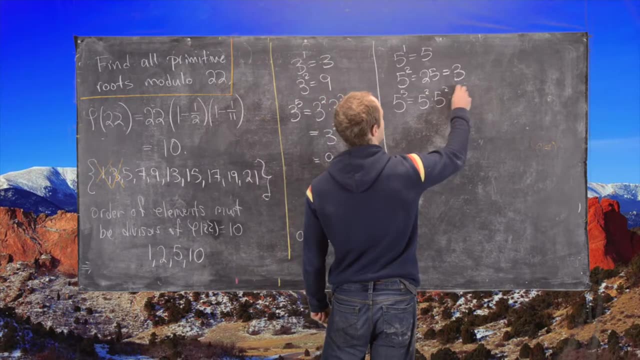 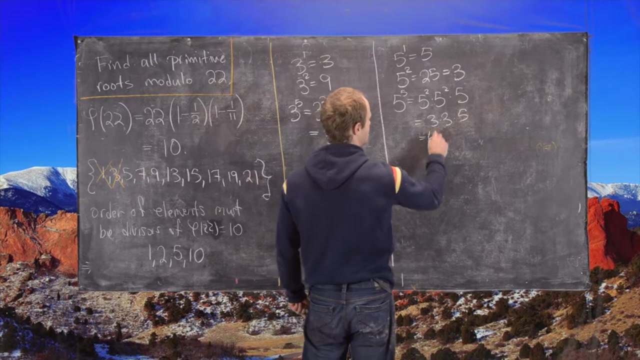 3. Great, Then 5 to the fifth is equal to 5 squared times 5, squared times 5. so notice, that's equal to 3 times 3 times 5, which is again equal to 45, which is congruent to 1. 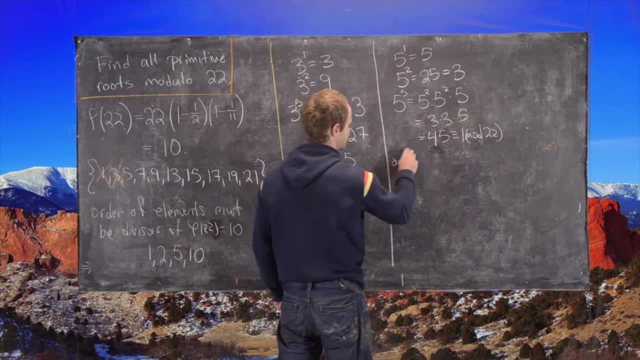 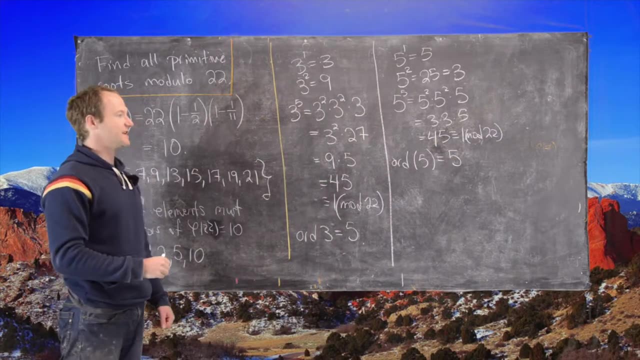 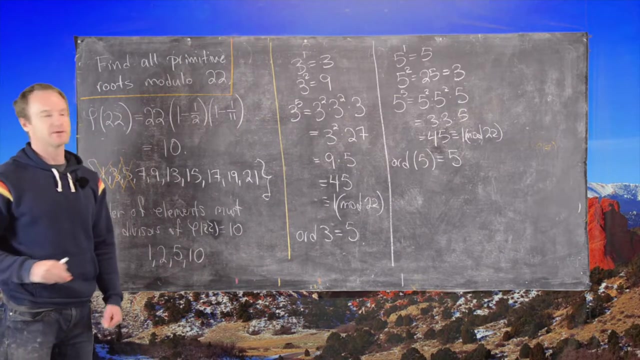 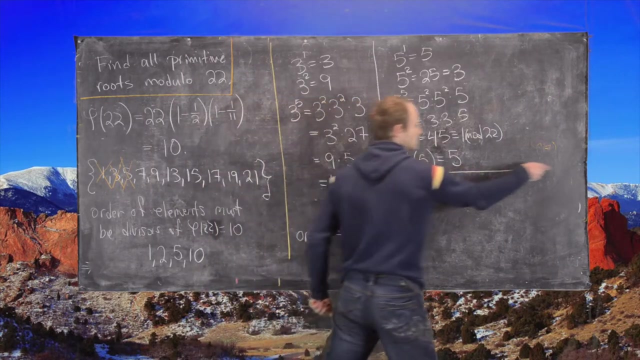 mod 22, which tells us that the order of 5 is equal to 5.. So, in other words, 5 is also not a primitive root. So we can cross 5 off from being the possibility of being a primitive root and let's move on to the next one. So the next one will be: 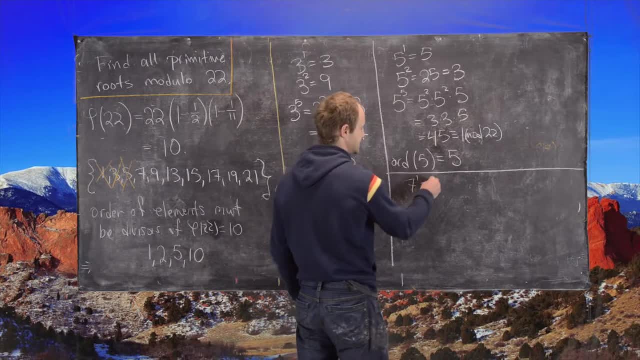 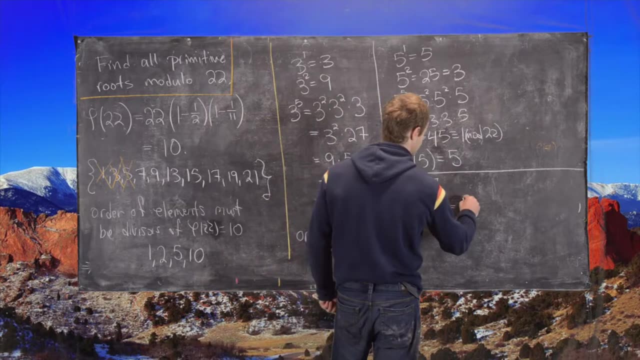 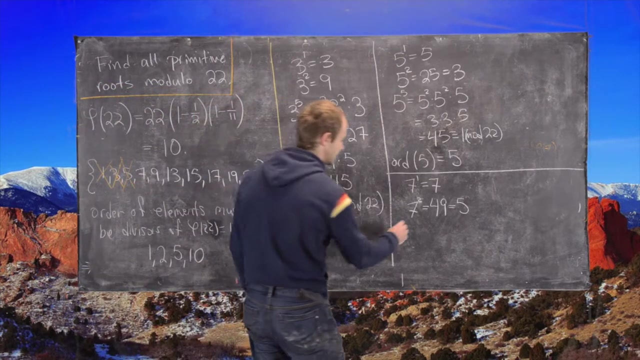 7. so we'll take 7 to the first. power is equal to 7. 7 squared is equal to 49, so 49 is equal to 5, because it is 5 more than 44. now 7 to the fifth will be equal to. 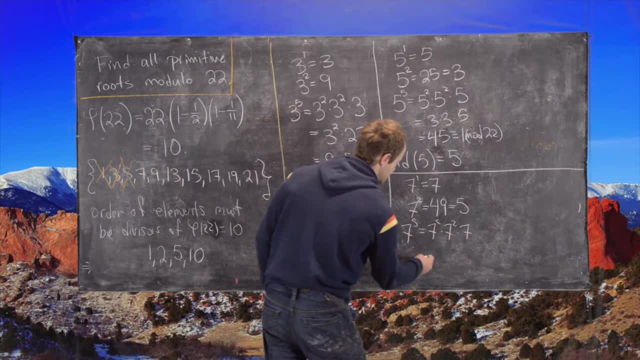 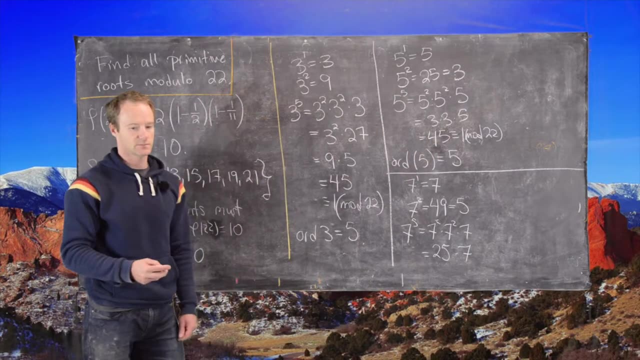 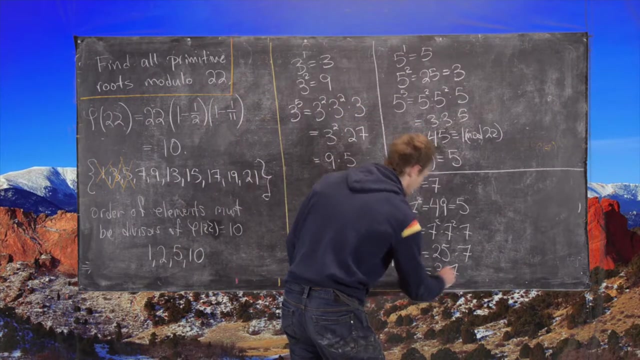 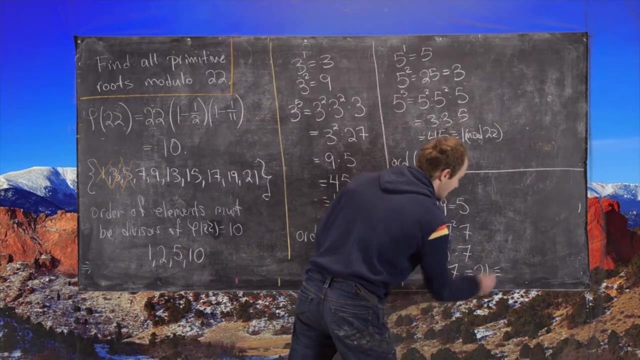 7 squared times 7 squared times 7. so let's see that is 25 times 7.. Good, But notice that 25 times 7 is the same thing as 3 times 7, because 25 is the same thing as 3, and so now that's equal to 21,, which is not. 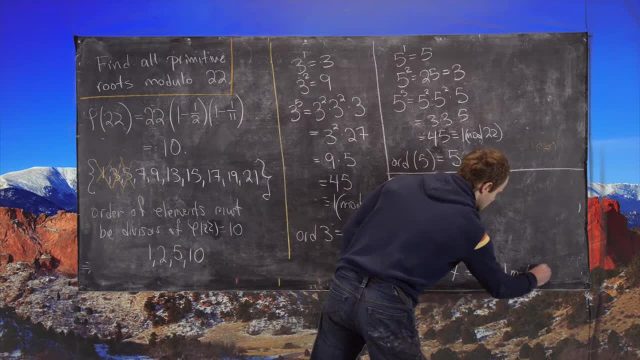 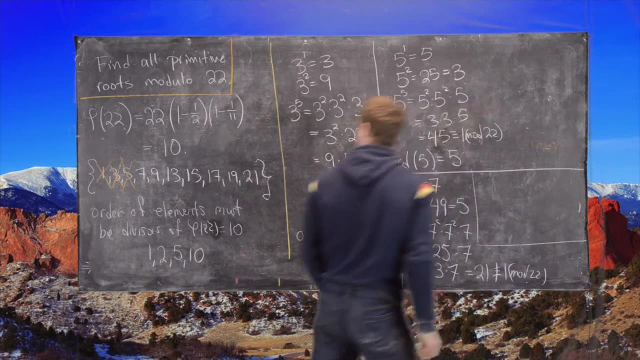 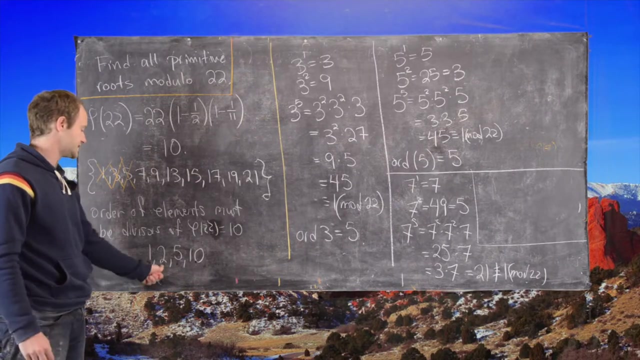 congruent to 1, mod 22.. Okay, good. So what that tells us is that recall that the only possible orders are 1,, 2,, 5, and 10.. So we've shown that the order of 7 is not 1,, it's not 2,, it's not 5,. 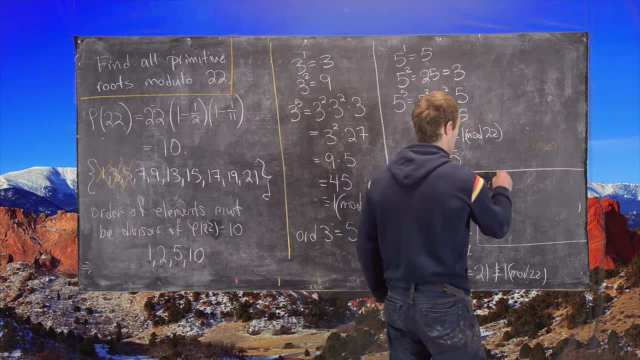 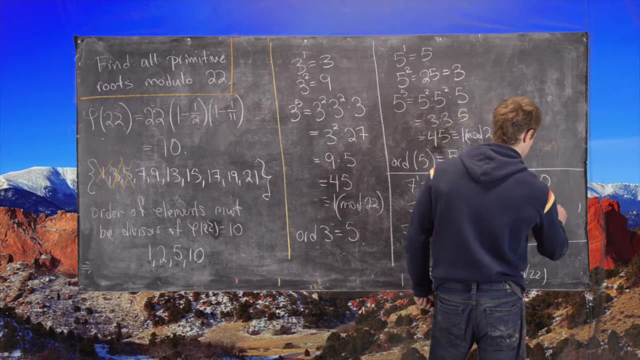 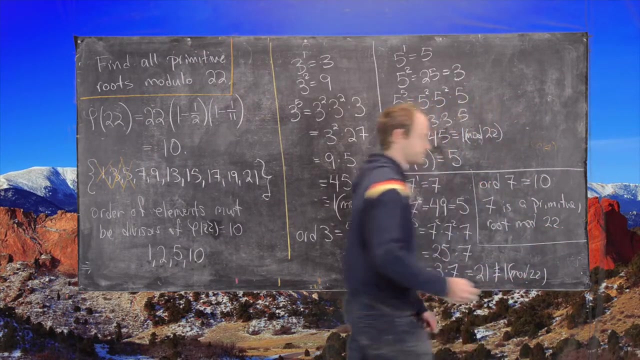 so it must be 10.. So we can write: the order of 7 is equal to 10.. In other words, 7 is a primitive root mod 22.. Okay, good, So I'll clean up the board, then we'll calculate all the rest. 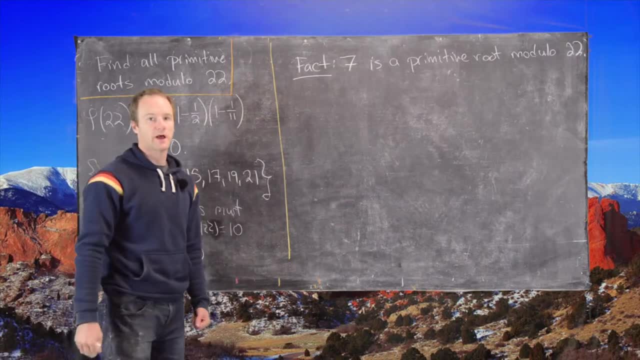 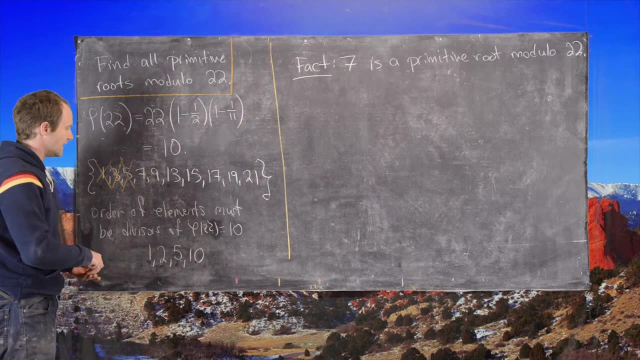 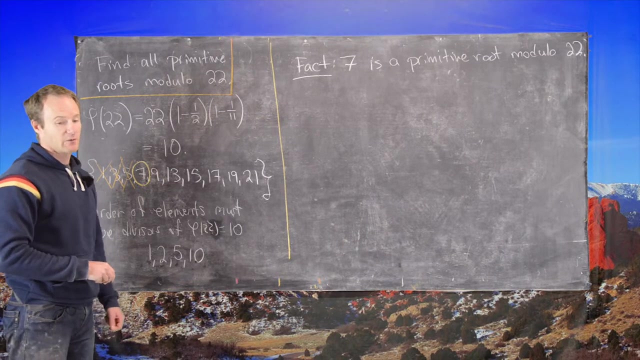 of the primitive roots, modulo 22.. Okay, so previously we had determined that 1,, 3, and 5 were not primitive roots- mod 22, and then we also determined that 7 was a primitive root- modulo 22.. So now what we want to do is calculate the rest of the primitive roots, modulo. 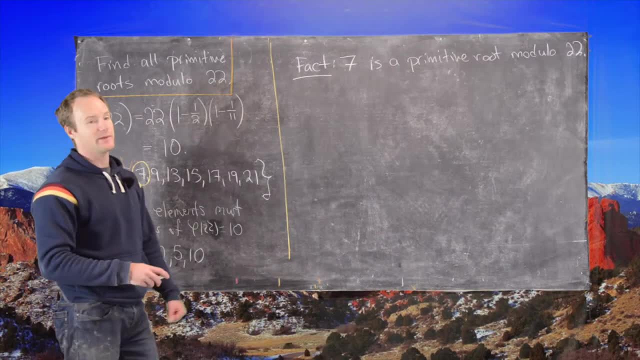 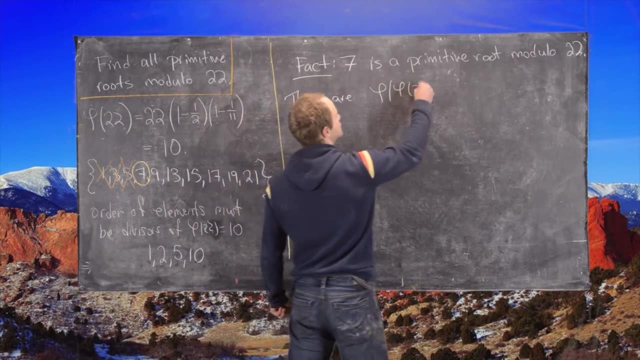 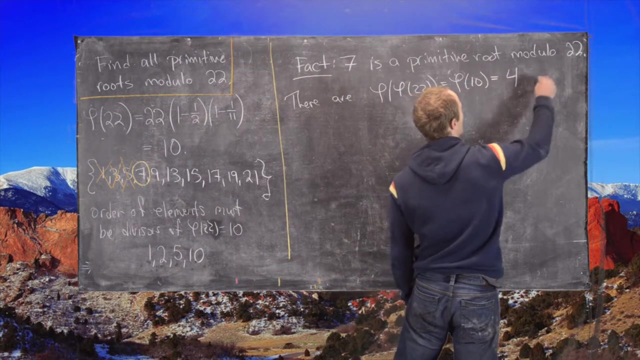 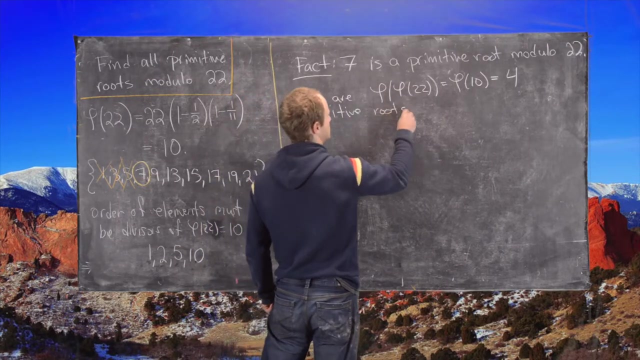 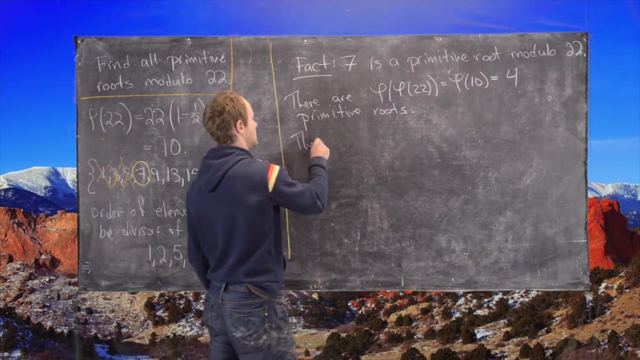 22,. and first let's check how many we expect. So there are phi of phi of 22,, which equals phi of 4 primitive roots. Okay, great. So now let's determine what they are. So they are. so, by the proof of: 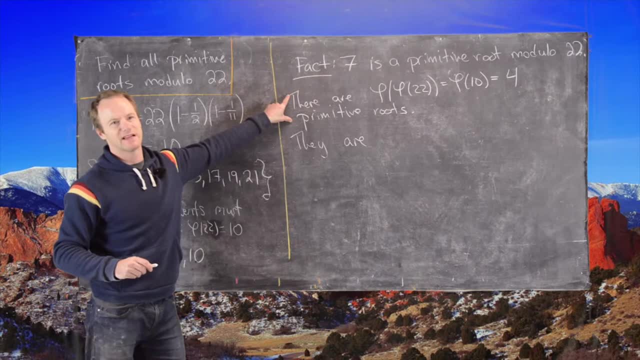 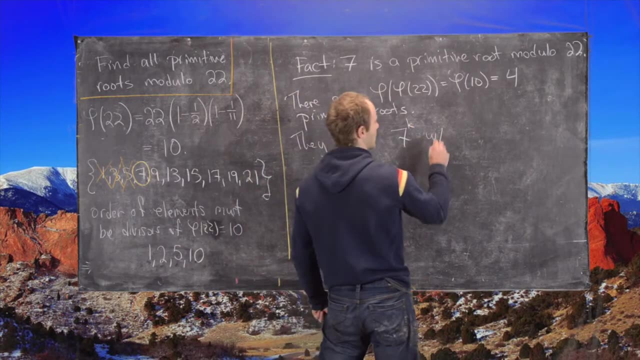 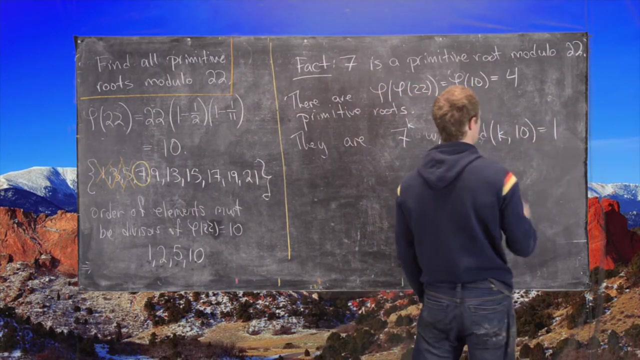 the general statement that we used. here we can see a strategy for finding such primitive roots, and so they are: 7 to the k, where the GCD of k and 10 equals 1. And here we're taking 10, so that's phi of 22.. Okay, great So. 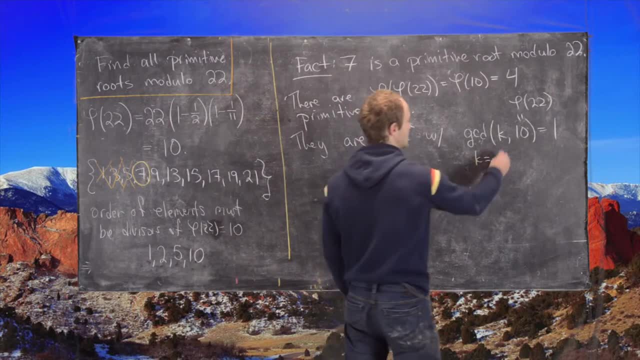 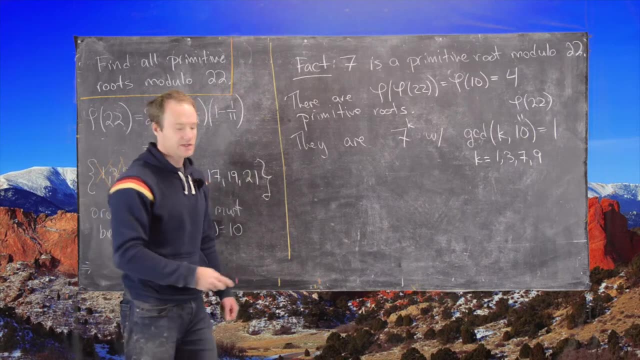 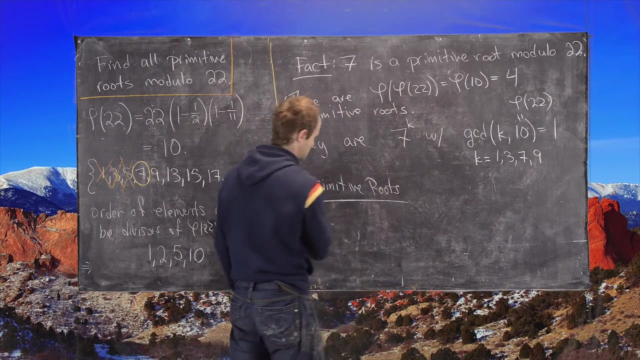 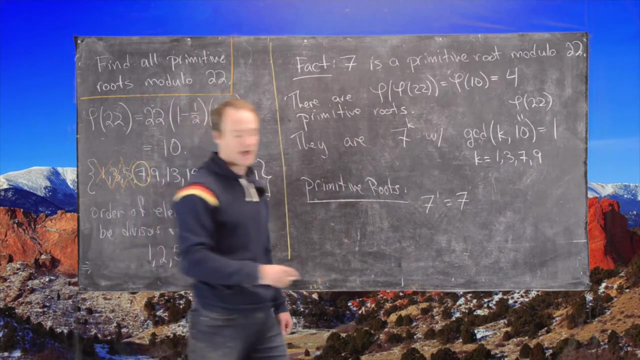 that tells us that k can be 1,, 3,, 7, or 9.. Okay, great. So that tells us. our primitive root list are as follows: So we get 7 to the first power, which equals 7.. We get 7 to the third power. 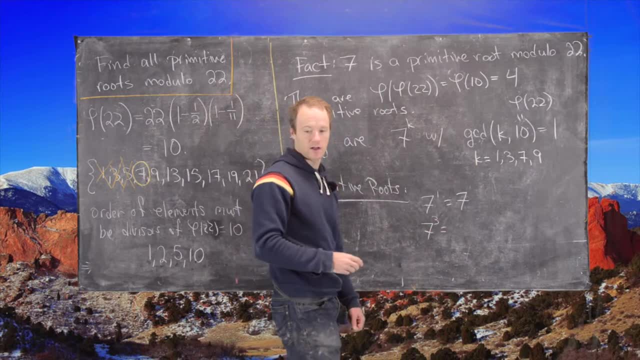 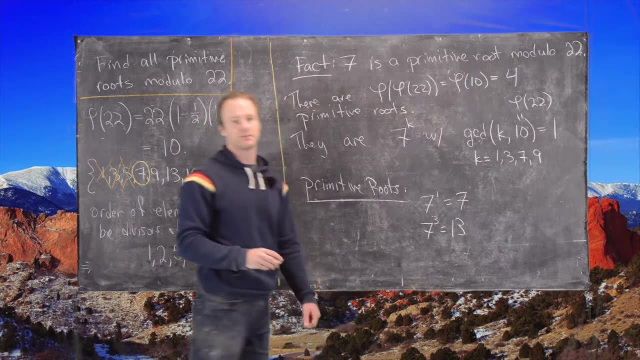 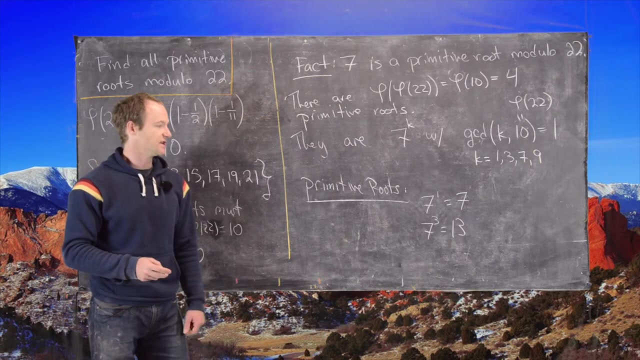 which equals. we get 7 to the third power, which equals 13.. So I won't do these simplifications, but you can use, like any strategy that we did in previous videos to do these simplifications. So 7 to the 3 is equal to 13.. 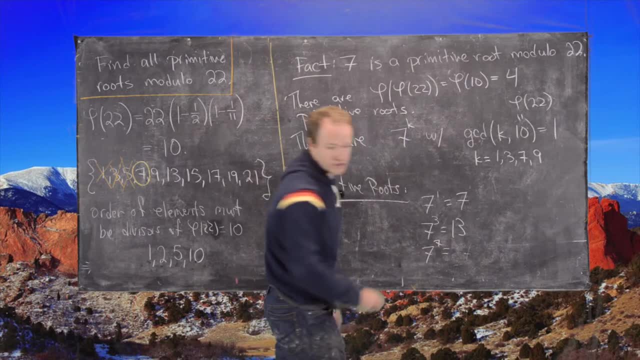 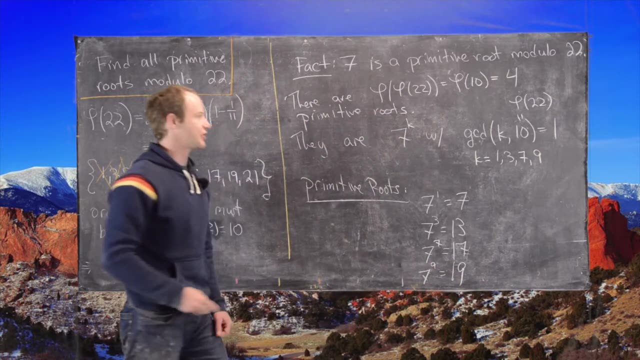 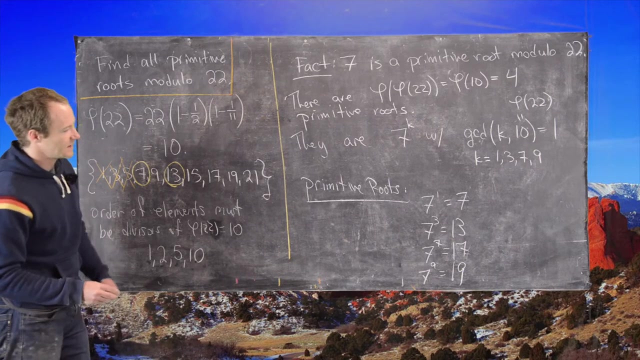 And then 7 to the 7,, which equals 17.. And then, finally, 7 to the 9,, which equals 19.. So those are your four primitive roots, modular 22.. So let's see, we have 13,, we have 17, and we have 19.. So 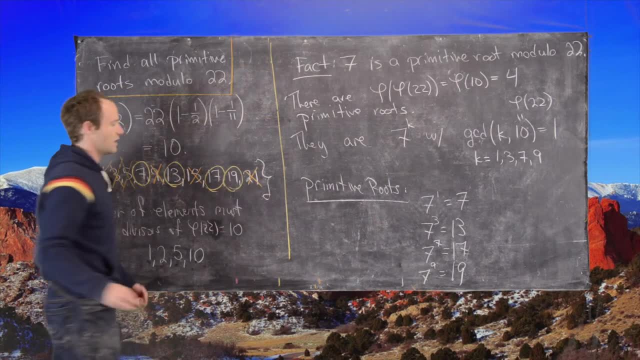 notice: we don't have 9,, 15, or 21.. Those are all not primitive roots. Okay, so that's the end of this example.